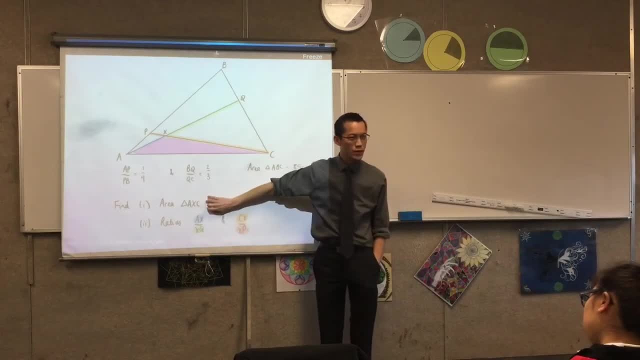 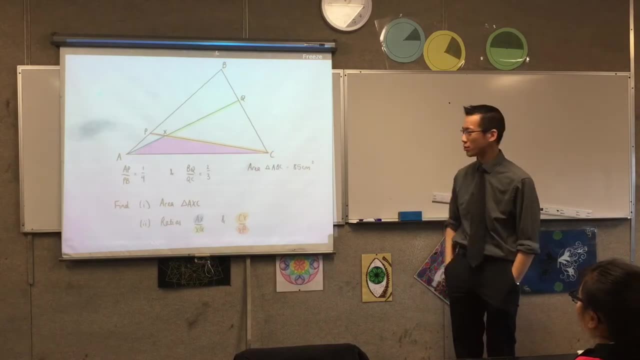 to measure any of them. I mean, as an example, how do we usually work out the area of a triangle? How do we usually do it? Well, at the moment we only really have one mechanism, which is base times height on two. So you'd need to know what this length AC is, You'd need to know its 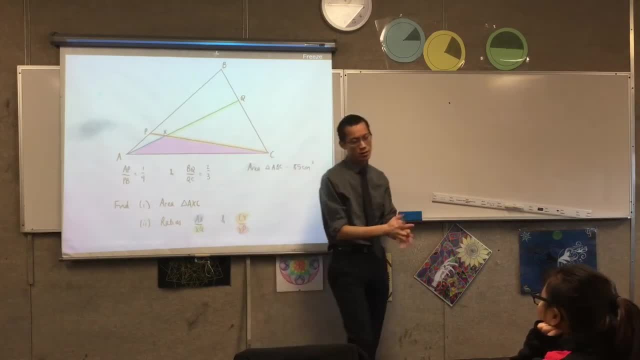 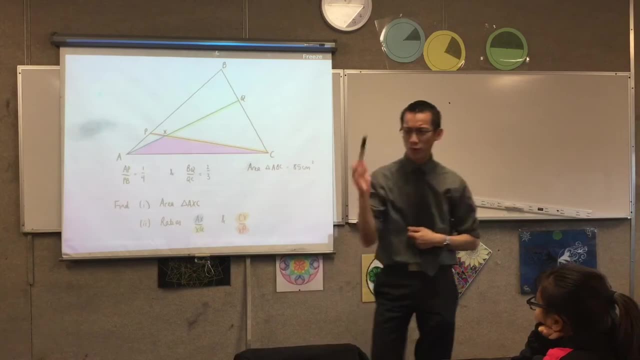 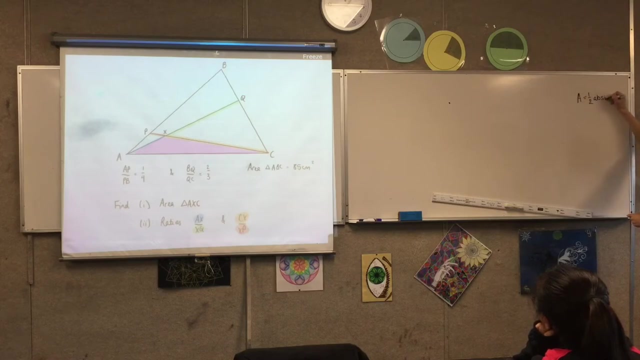 perpendicular height, or I suppose you could define anything as the base and therefore get the corresponding perpendicular height, But the point is you need to know some lengths. You will learn pretty soon that one other important way for working out the area of a triangle is using 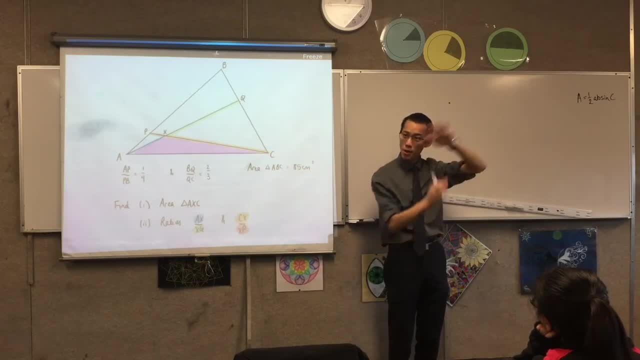 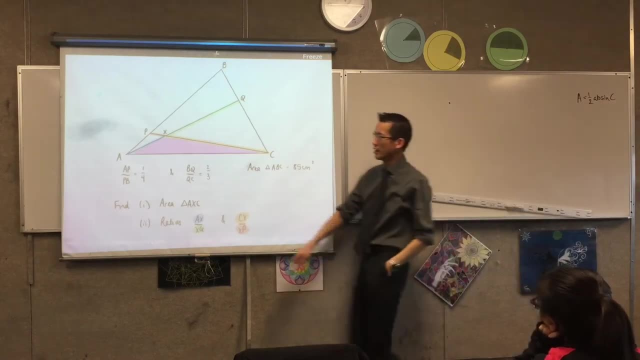 trigonometry If you have no base and perpendicular height corresponding to it, its equivalent to have two sides and an included angle. Do you know what those are Like? for example, if you knew what length AX was, length CX, and if you knew what this angle AXC was, you could use this and you could find out. 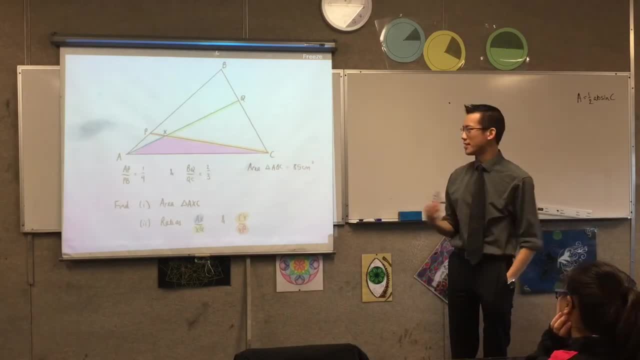 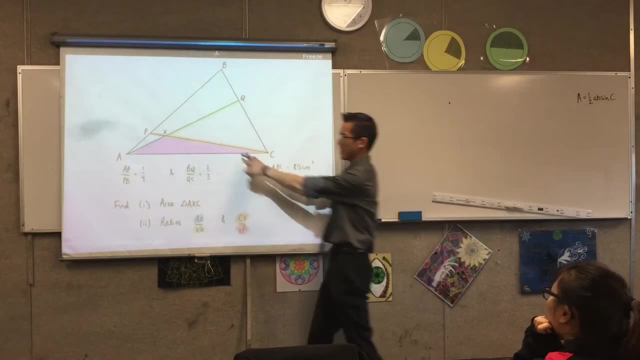 the area. Okay, But kind of the whole point of this is that this can vary about. This can be a different set of shapes and it might have a different set of angles or a different length down here in proportion to these two. So how do I work this? 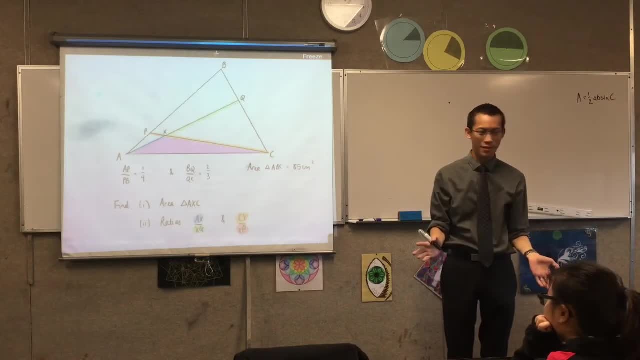 out this area without knowing any of those things. Okay, All I have is these ratios, So I want you to have this sort of settling in your mind. We're going to draw this diagram and we're going to work with it further as this. 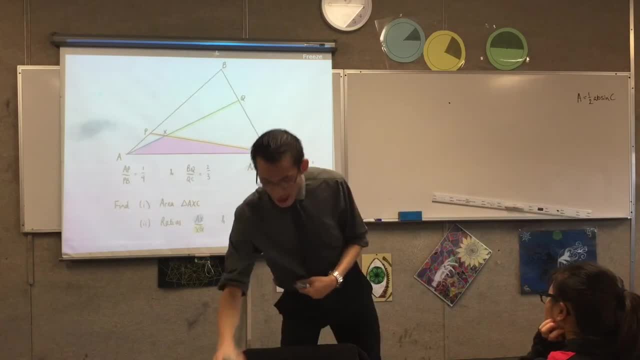 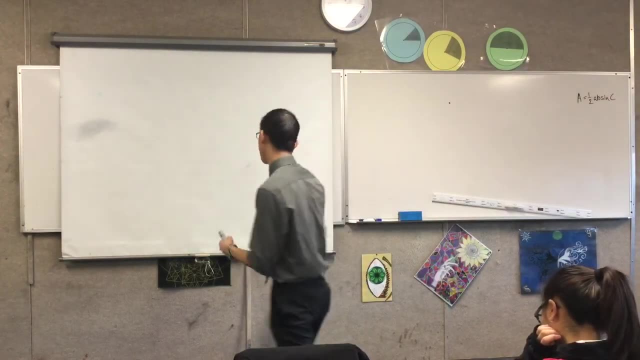 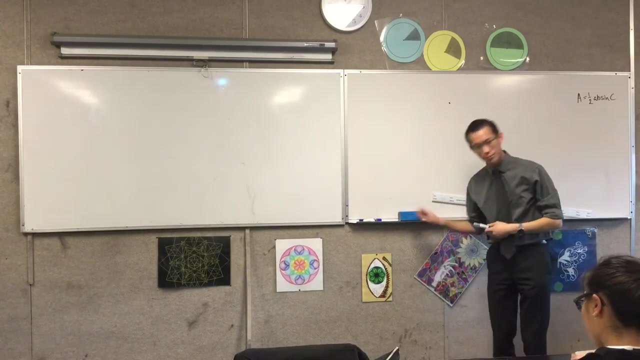 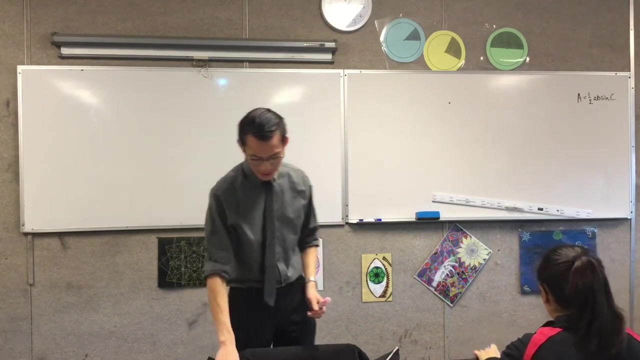 lesson progresses. But I'm going to put this away now And you can make the heading, if you like, of parallels. We're going to be drawing a whole bunch of diagrams and working out how to relate different areas and lengths together when all you have is ratios between them. So I've got- let me count it- one, two, three, four, Four, little. 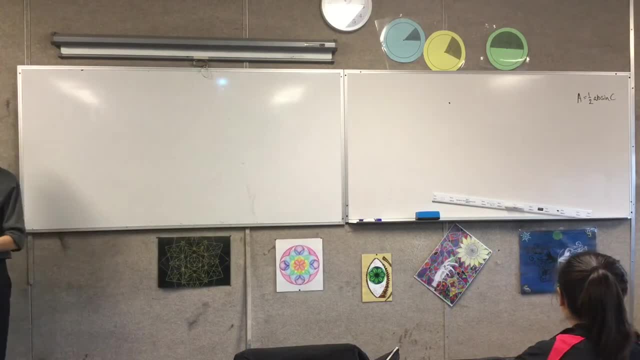 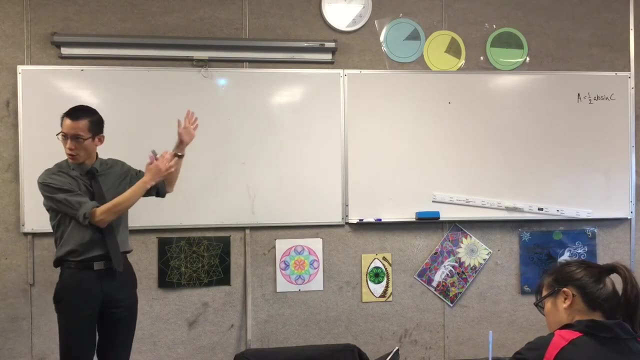 sort of theorems or properties for you, And again I'm going to blow through them fairly quickly because I know you've seen the early ones before, So this is more just a little bit of a puzzle. Okay, have it in your mind so that it's sort of like fresh as you go through the challenging. 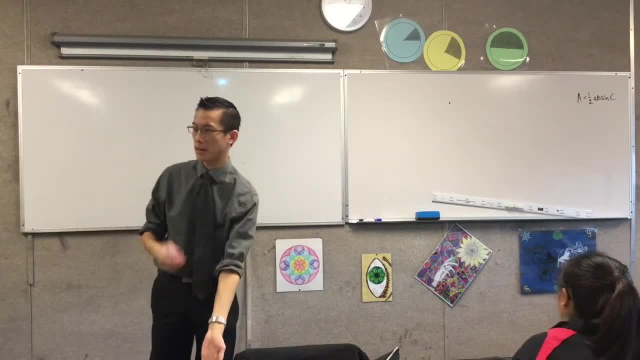 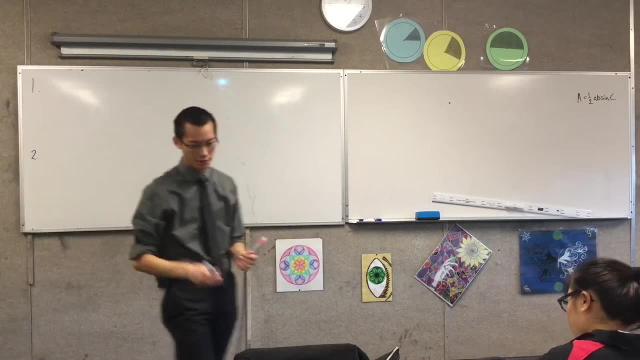 questions: Four little properties, and I'll give you the wordings for each, But the most important thing is the diagrams that you draw with each of them. Okay, So let's do the first two as a pair, because they kind of fit together. 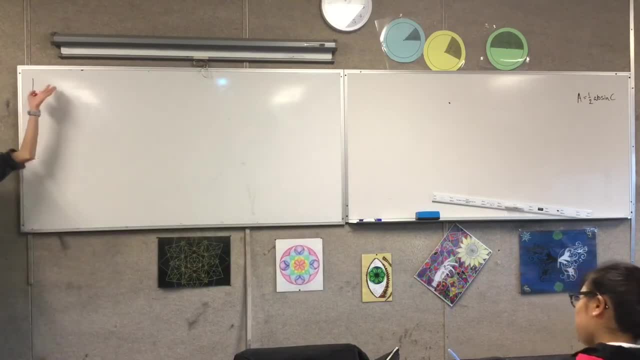 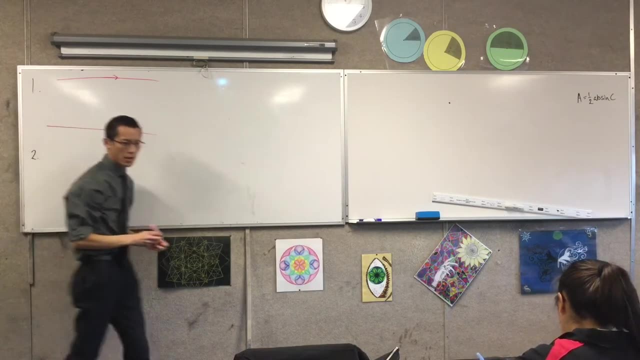 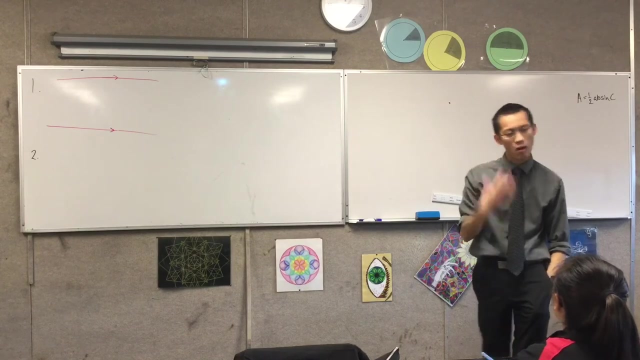 Would you draw for me please For each of these two properties? I'm about to show you a pair of parallel lines And I will just also show you the first two as well. You know, if you have colours here, if you have colours like colour pencils or highlighters or colour. 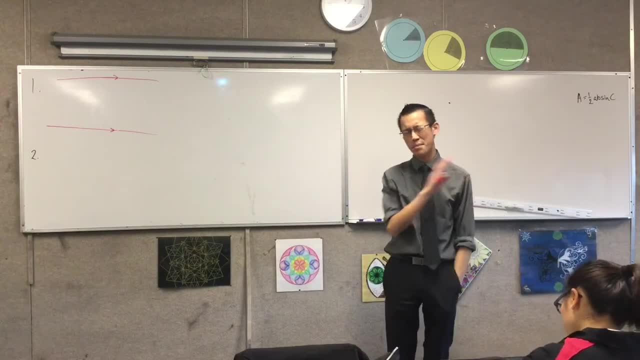 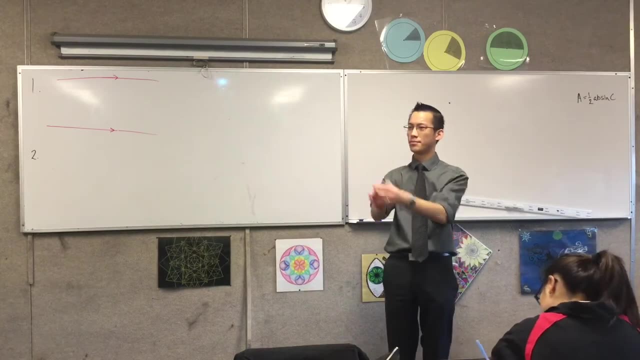 pens or anything like that. there'll be enormous use to get them out as many colours as you possibly can In geometry. geometry is so much a problem of vision- right, If you can see a question properly, if you can see through the maze of lines to what really matters. 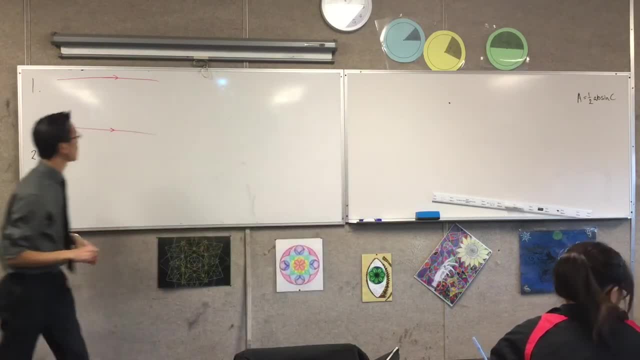 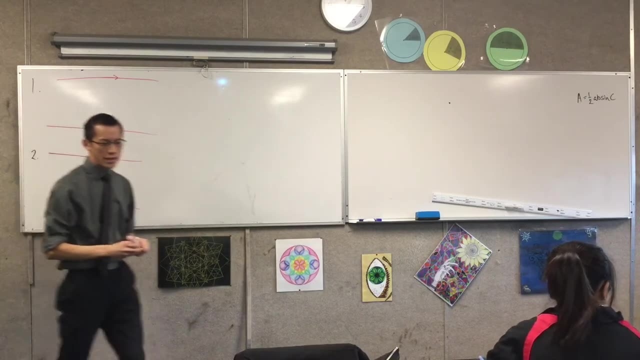 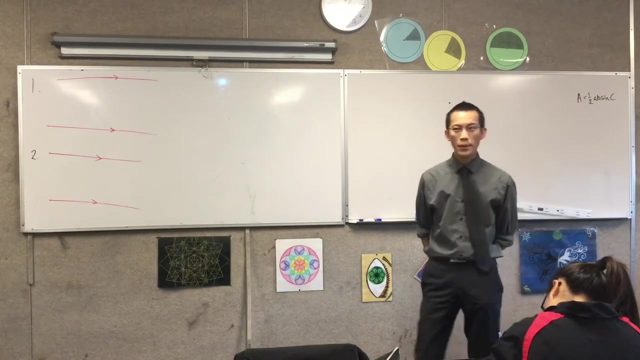 then you can often solve a question very, very quickly. Okay, so I'm going to use quite a few colours today. So, like I said, For these two properties, you'll need a couple of parallel lines for each Right property, number one. 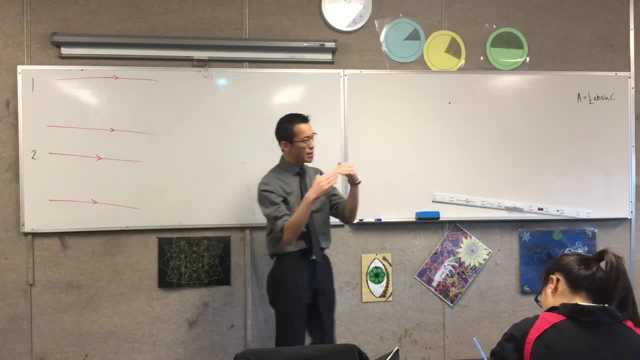 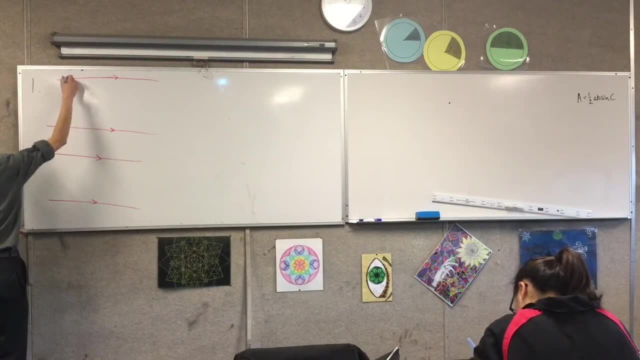 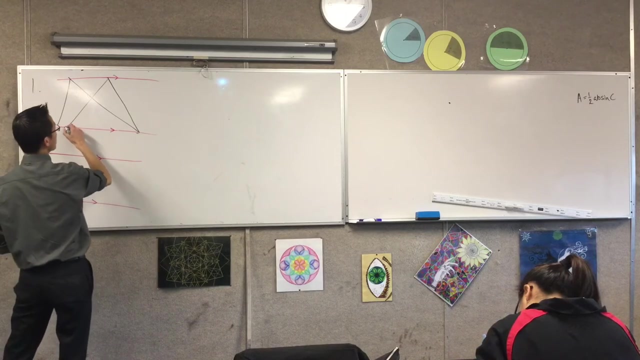 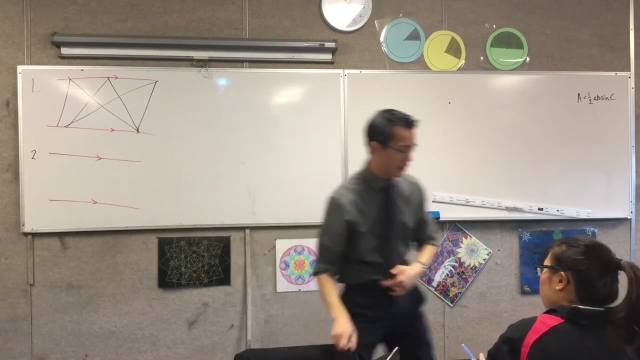 If you've got a pair of parallel lines and you create a set of triangles between those parallel lines, Triangles like this: Okay, so if you have a look at these right, What I've got is a set of triangles that are bounded between these parallel lines. 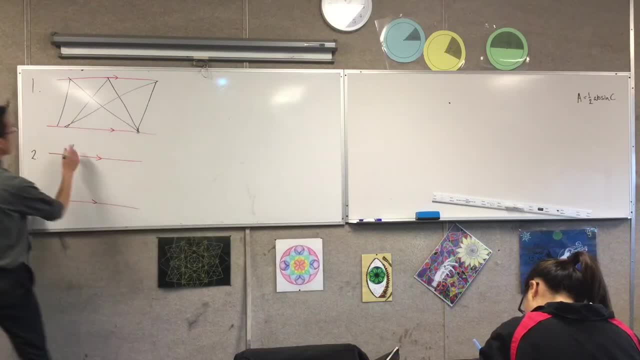 But, importantly, here comes my first other colour: Each of them. this is a bit off, let me fix that one. Each of these triangles is not only between the parallel lines, but they also all share the same base. Let me pop that in here. 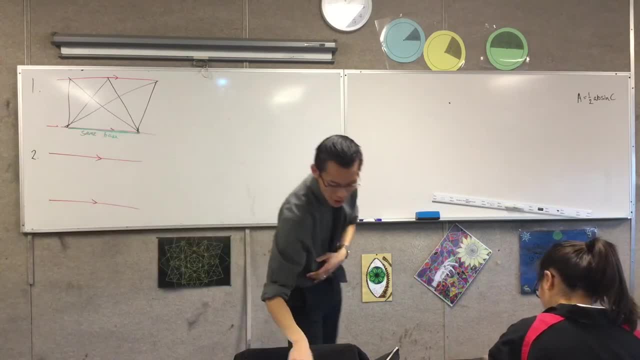 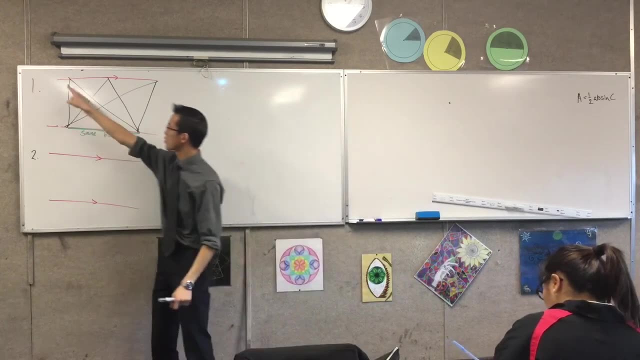 Okay now, because they're all between the same set of parallel lines. the distance between parallel lines all the way along, like the distance from here to here, the perpendicular distance between one parallel line, the top one and the bottom one, is always the same. 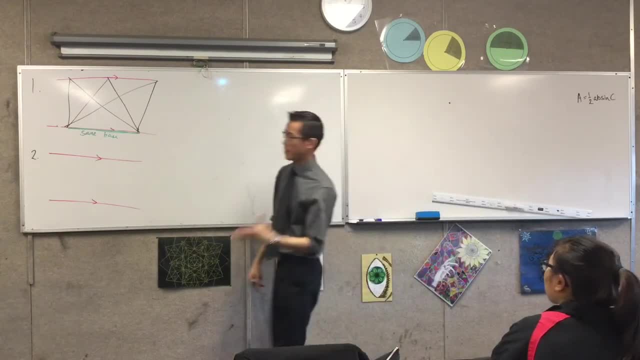 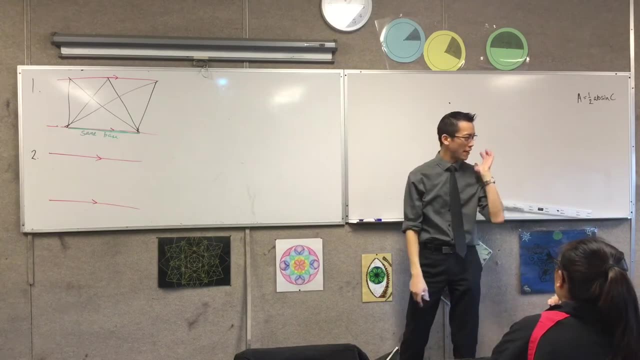 Every single time. okay, If you like, you want to think about it this way, I can construct a set of rectangles all the way along here. they're all at the same height. okay Now, because if I did that between these parallel lines, I'm always going to get that shape. 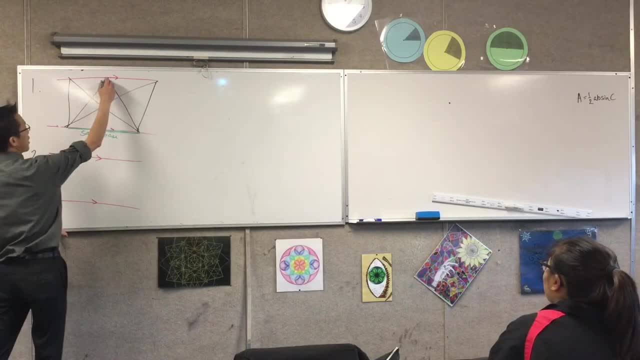 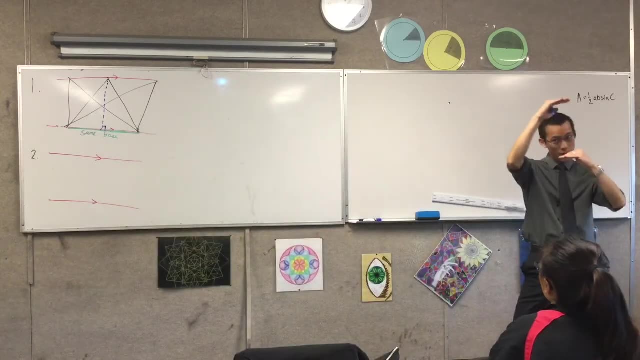 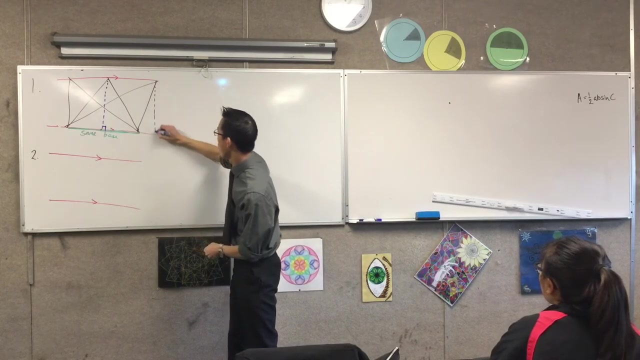 For example, If I put in the perpendicular height of, say, this triangle, You can see, because that line is perpendicular between those two parallel lines. it's always going to be perpendicular, no matter where I move it. So, for instance, I could move it over here. 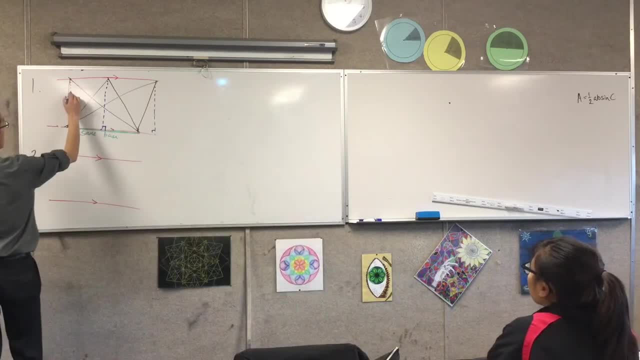 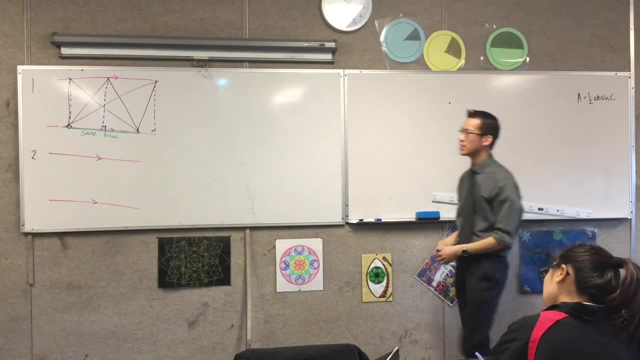 And it would still be perpendicular. Or I could move it inside here, And it would still be perpendicular. okay, Now, the reason why I've drawn all three is because now it kind of makes clear to you if you look at one of these triangles. you remember, at the beginning I asked you: 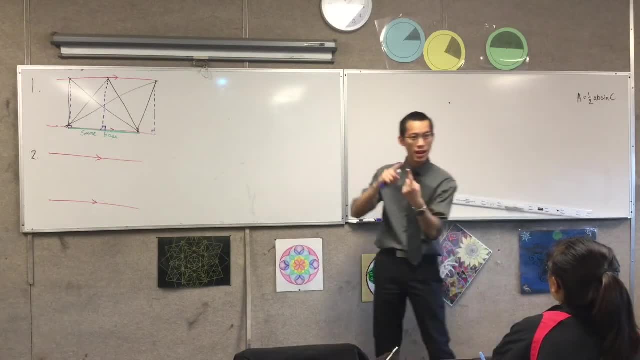 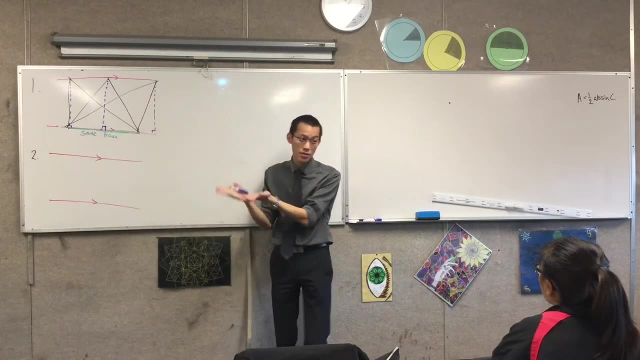 how do you work out the area of a triangle, right? Well, at the moment, you need two things. You need a base- You can see these all have the same base- And you also need the perpendicular height, And these all have the same perpendicular height. okay, 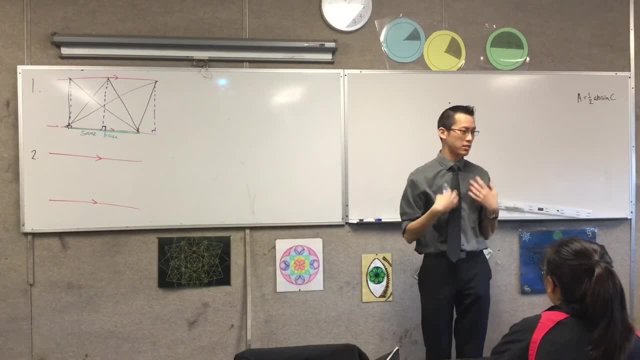 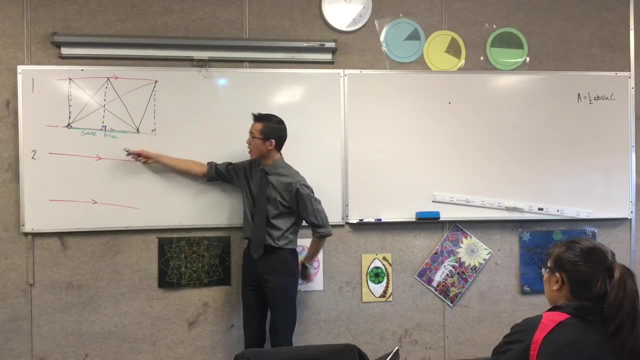 So here comes the wording of the property. I'll say it once and then I'll say it again slowly, so you can write it down if you'd like. But the important thing is the diagram. Triangles on the same base. Triangles on the same base. 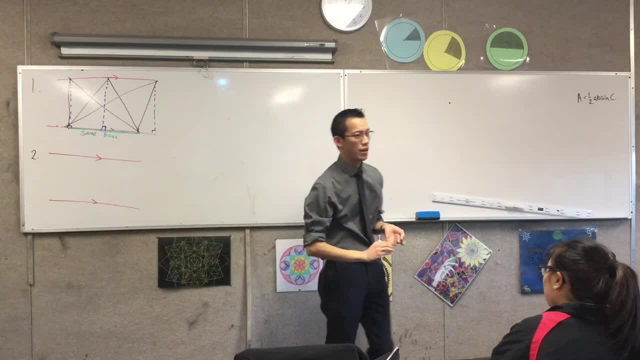 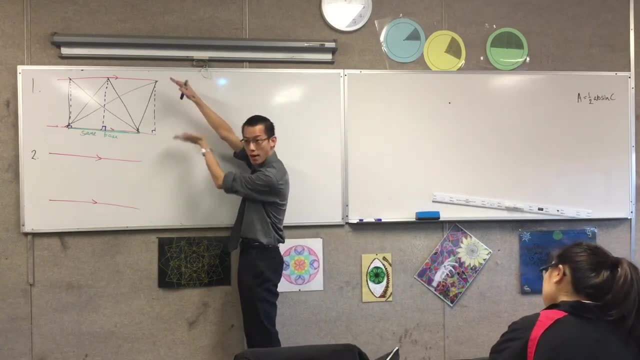 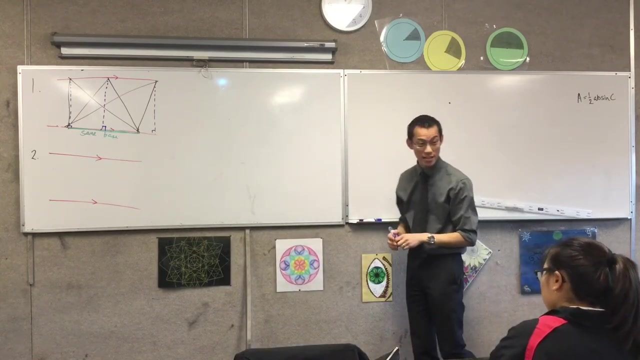 Between parallel lines Are equal in area. That's it. It's not crazy. Triangles that have the same base Between parallel lines Have equal area. That's all that's there, okay, And I kind of think the diagram says that for you. 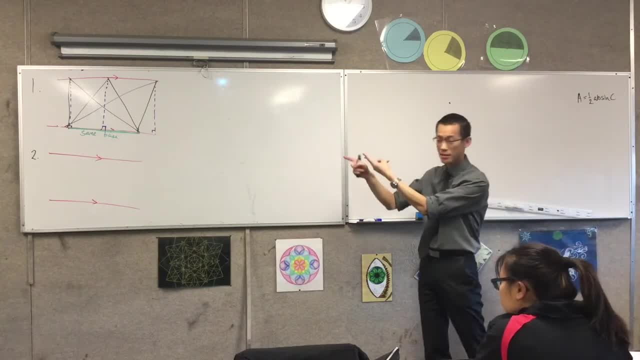 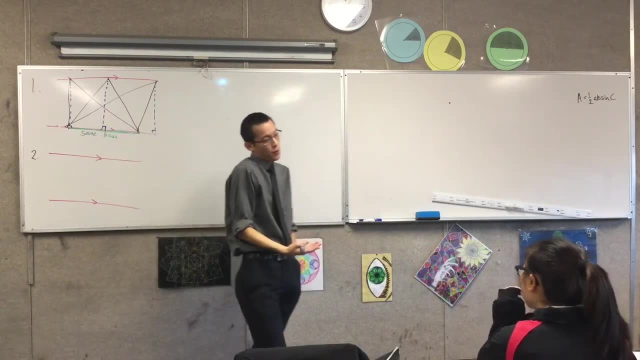 Again, they're all triangles, They all share that same green base down there, And because they're between those parallel lines, that's what gives them all the same perpendicular height. So therefore, same base, Same perpendicular height, Equal in area. 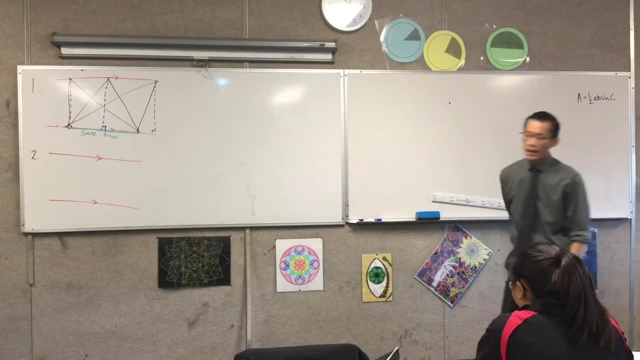 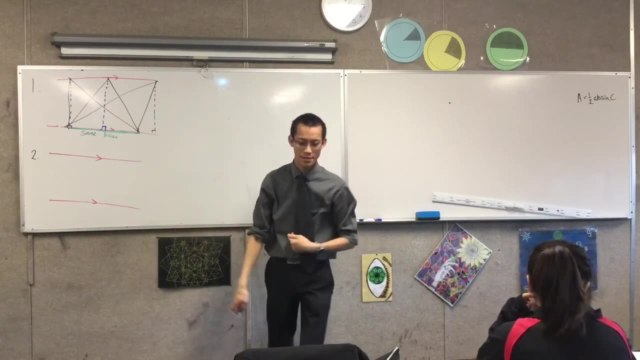 Okay, There's the first idea, And the second idea is kind of like that, but just slightly twisted. okay, If I stay between these parallel lines. okay, Let's draw a new pair of triangles now. Sorry if I do it like this. 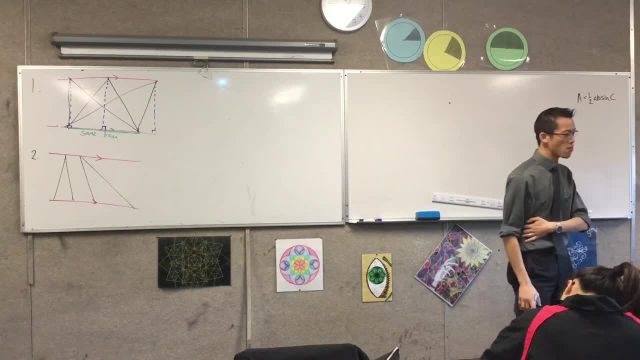 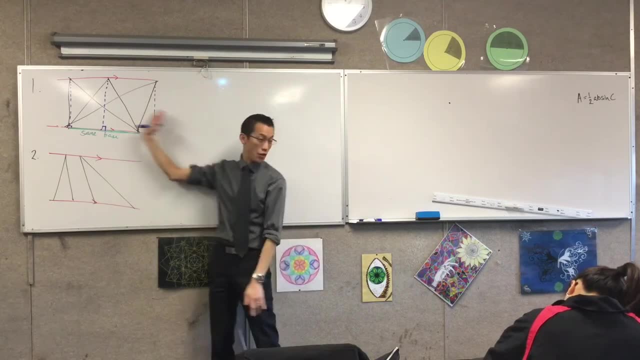 Okay Now, unlike in our first case, where you've got triangles on the same base and between the parallel lines, So therefore they're all the same. They're all the same. You can clearly see these two triangles, not the same. 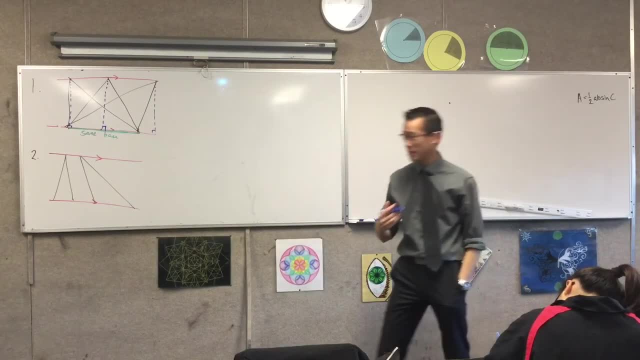 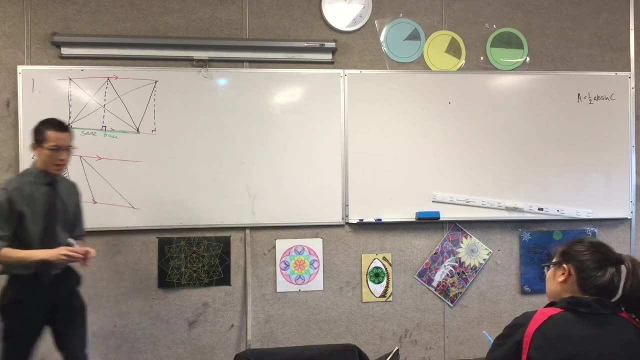 Are they? They're not the same, And so I'm going to colour them a little bit differently to indicate that. So over here, I've got this skinny guy on the left, So let's do human blue, And then off on the right, we have this one that's slanted over a little more. 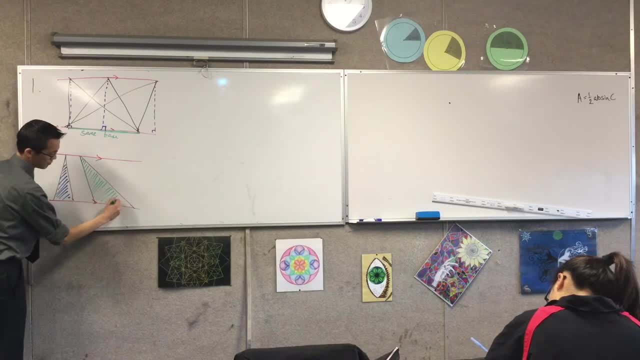 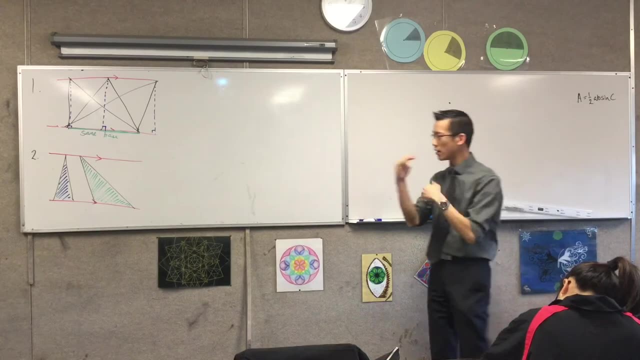 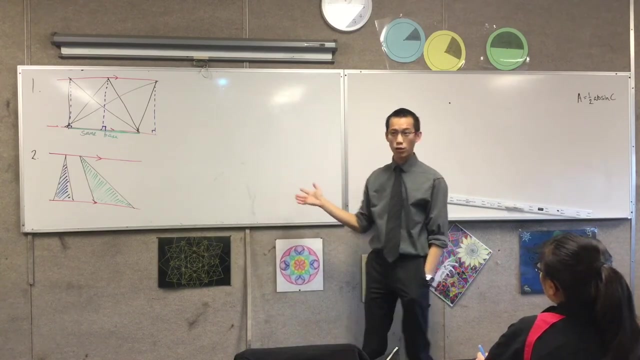 A little bit of a choose angle in it. Okay Now, in this case, because I'm still between parallel lines, even though these triangles are very different, there's still one feature- and I mentioned it in the first property, that these two triangles share. 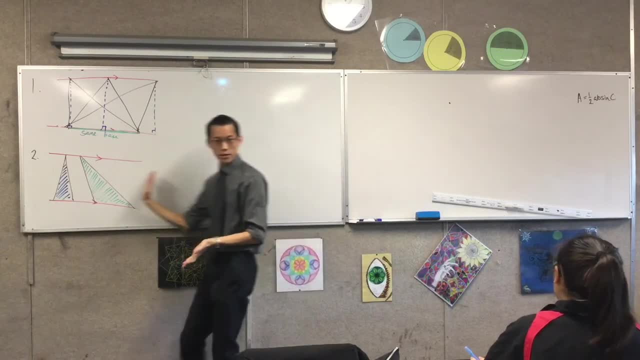 What's the property they share? The perpendicular height. The perpendicular height. Very good, That's what those parallel lines are doing for you, right? Every single triangle, wherever you draw them, I could draw them all the way over here- same perpendicular height, okay. 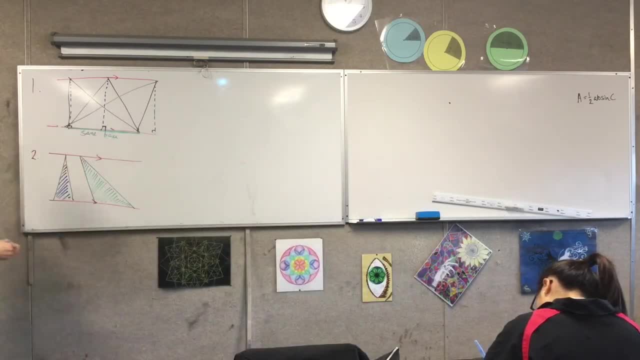 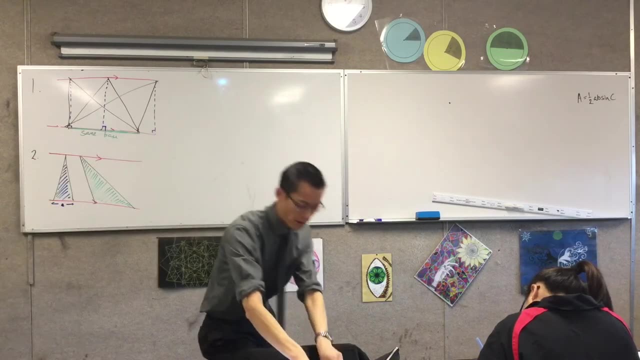 So all that's different between these two is their bases. Now, if I just like name these bases, let's call this length over here A and we'll call the base of the other one. very originally, mathematicians always known for that kind of thing. 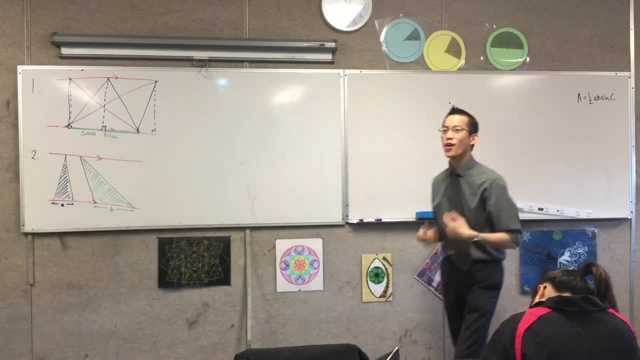 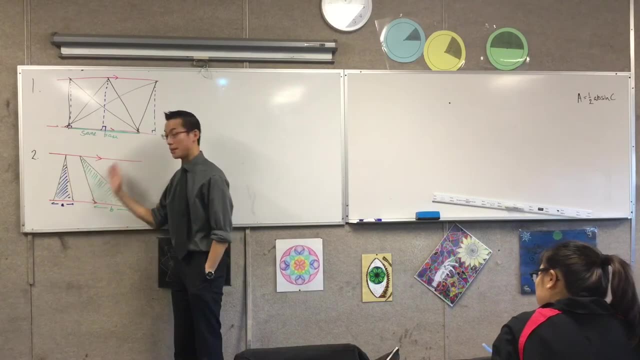 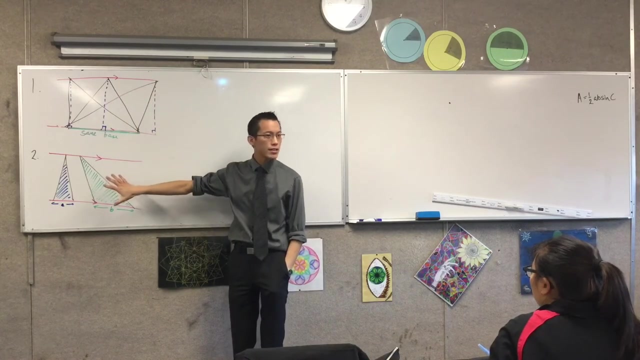 B. Okay, If the ratios of their bases are A to B- because the only other measurement that is different is the perpendicular height, but that's equal in both cases- then here the areas are all the same. Here the areas are not the same. 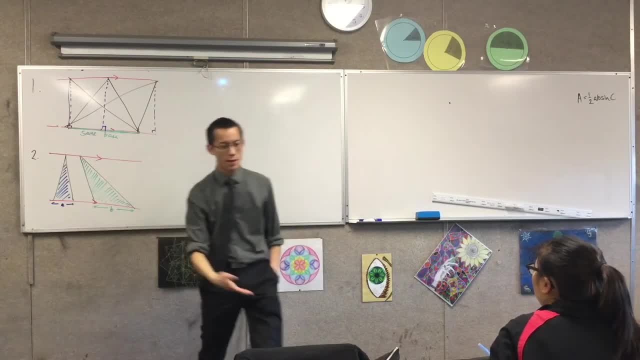 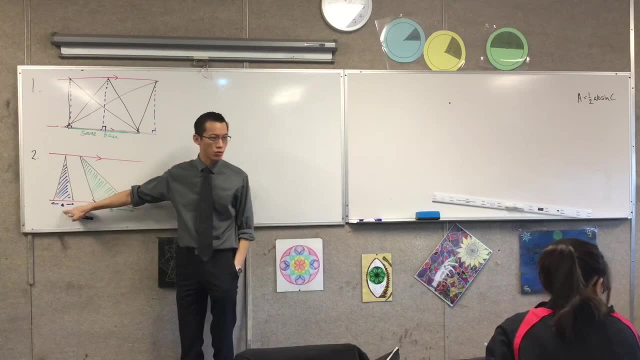 but they're in this ratio. Can you see that? So, for example, if I actually called the perpendicular height of this H, as we often do, okay, what would the area of this actual triangle be? The blue one? Yeah, very good. 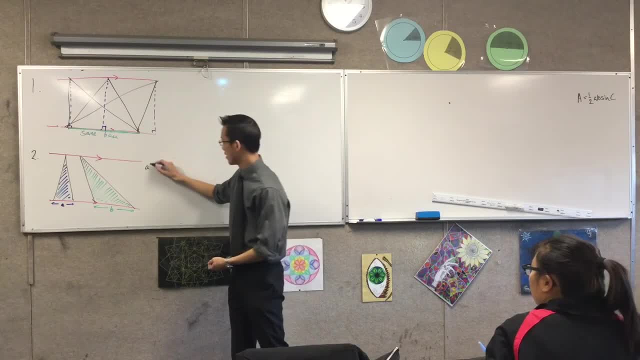 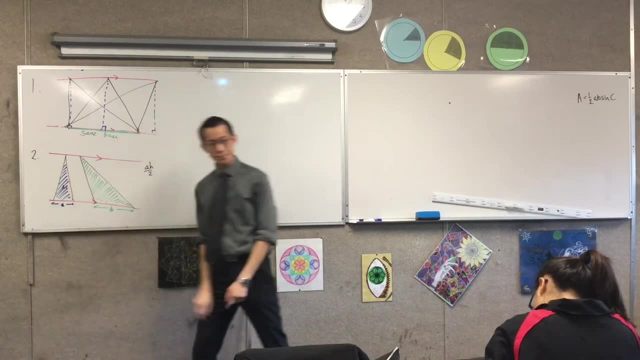 It's going to be the base, which is A times the height on 2, right. So that would be this area over here. I'll call this A1.. This one over here A2, everything will be the same, except I have a different base, right. 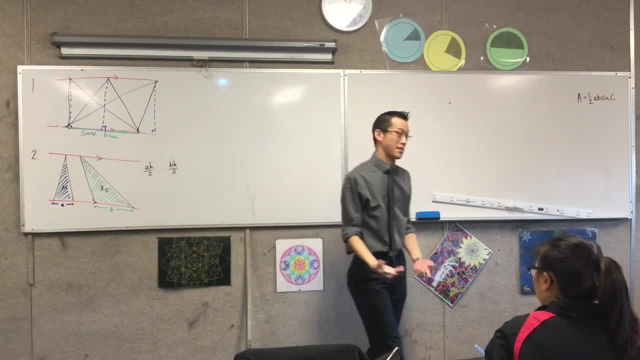 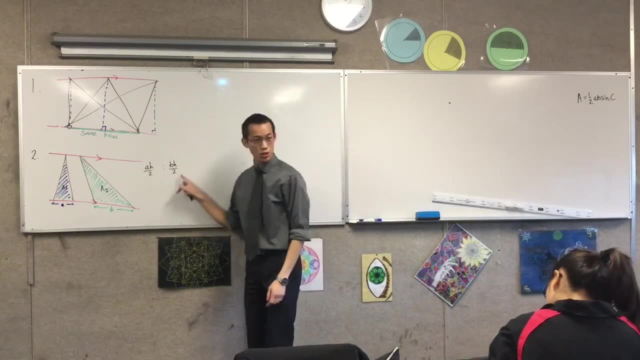 It's going to be base times height on 2, except my base this time is called B. Okay, And you can see here whatever H is, it's just a positive number. This 2 here is another positive number, So just like any other set of ratios.